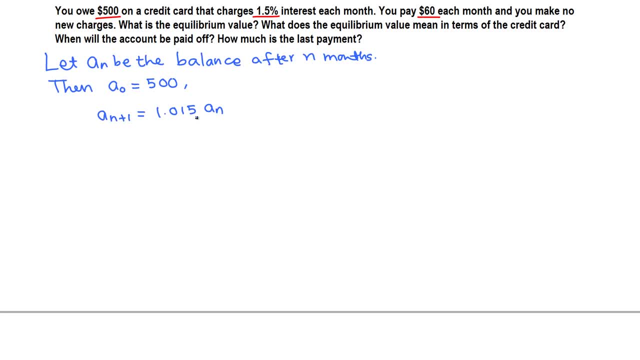 so 1 plus 1.5 percent, that's 1.015 an, and you'll be 60 each month. that means minus 60.. Okay, this is for. n equals 0, 1,, 2, 3, etc. Now we need to find the equilibrium value. okay, then the. 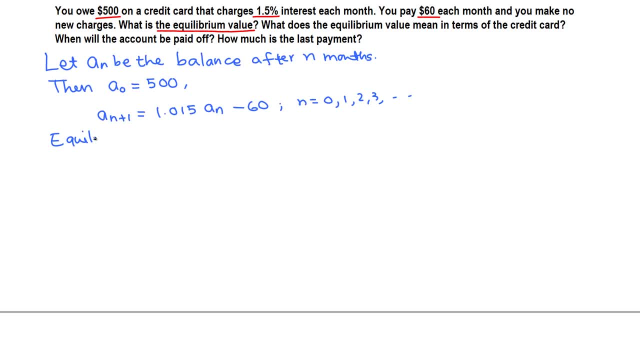 equilibrium value is found by the following formula: equilibrium is given by B over 1 minus r. So in this question this is B and this is r, which happens to be bigger than 1. so equilibrium value is B over 1 minus r. that is negative, 60 over 1 minus 1.015.. 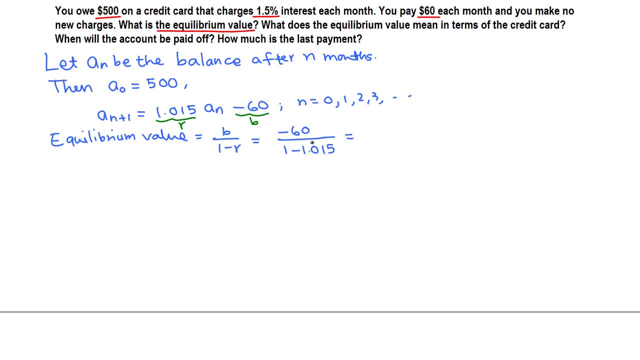 Now use your calculator and it comes out to be 4,000. okay, Okay, $4,000. and since r is now, we need to explain. what does this mean? okay, so what does the equilibrium value mean in terms of credit card? so the initial balance is 500 and the 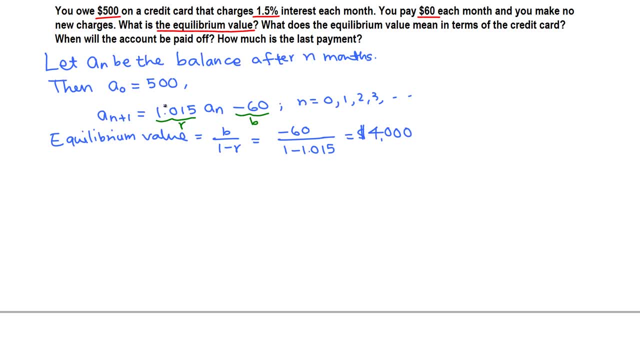 equilibrium value is 4,000, but r is bigger than 1. so since if we take absolute value of r in in this case is the same thing, which is one point zero, one five which is bigger than one, this equilibrium value is unstable. the equilibrium value 4,000 is unstable. that 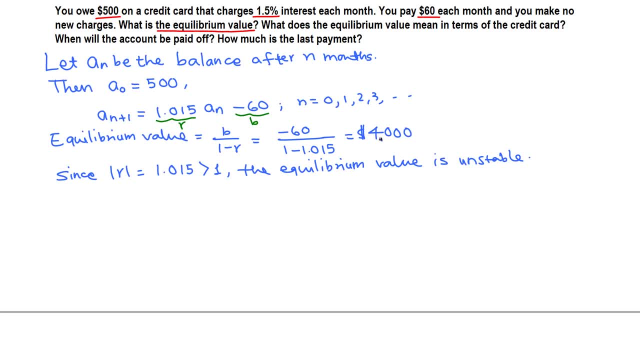 means all the values want to go away from 4,000, eventually away from, since initial balance is five thousand 500. so we kind of have kind of like this way: here is 500 balance and 4000 is initial value, so eventually that's the equilibrium value. everything stays away. go away from this line. 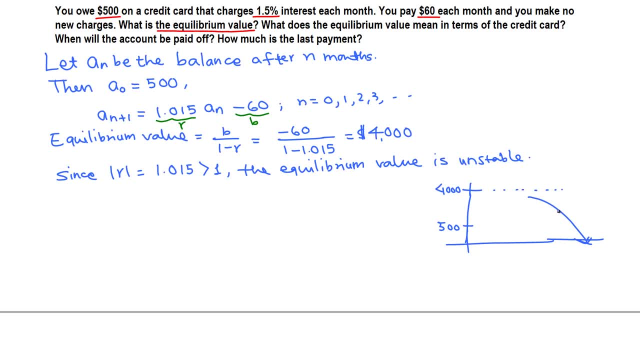 so eventually this goes to these curves go to negative infinity. that means the balance will be zero at some point. that means the credit card can be paid off. okay, if this initial balance is bigger than 4000, then they would go up. that means we can never pay the credit card off. 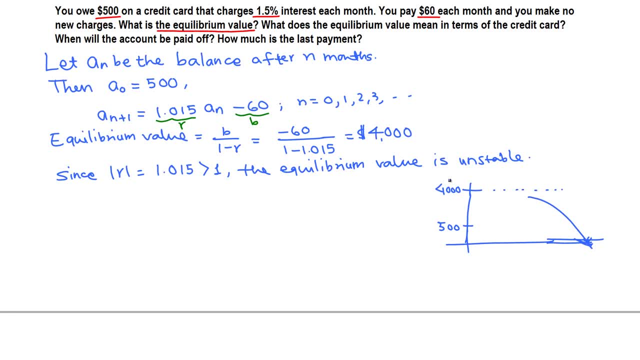 so in this case we can pay unstable and our initial balance A0 is. that's 500, is less than 4000 equilibrium value. okay, the credit card can be eventually paid off. can be paid off. okay, now we need to find when will the account be paid off. so we need to find this: 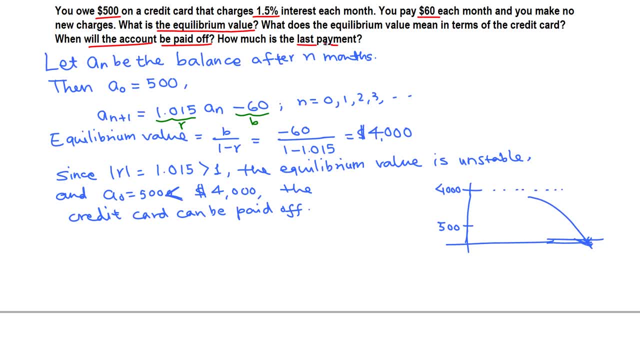 number of months and how much is the last payment? okay, so for we're going to use this dynamic system and take n equals zero, we find A1. that's the balance after first month. take n equals one, plug in here, we get A2. that will be the balance after second month. and let me do that using a calculator. 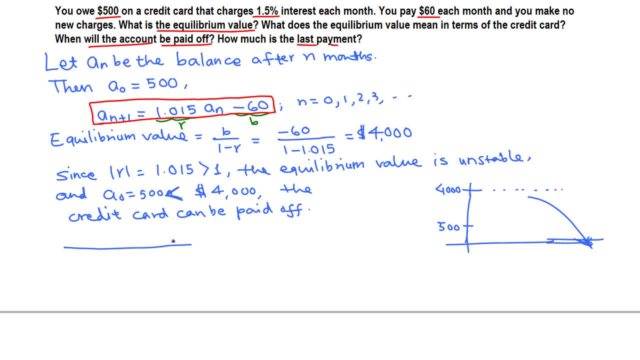 and will get the following: so n equals zero and corresponding a. so when N is zero, not zero, here let me write e, n values here. when n equals zero, that's A0, the initial balance is 500,. okay, after one month that means taking n equals zero, and that's the balance after slowly. okay, after one month, that means taking n equals zero. that's initial balance: 500. okay, after one month that means taking n equals zero and the balance domestic value here. well, hey, when n equals zero is zero, then this is the begins of initialzener B0, c if it first line scale means starting at substation more than here. 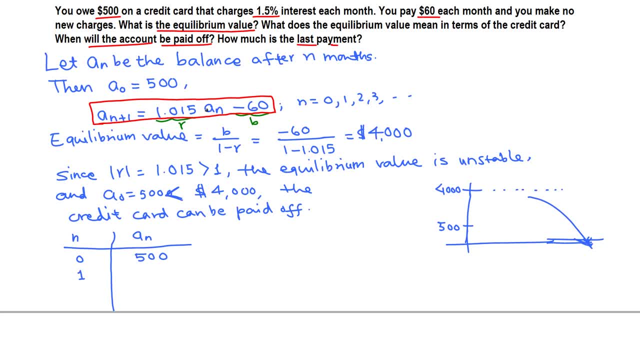 and plug in here 1.015 times a0. a0 is 500 minus 60 and use your calculator, you get 447.5. take n equals 1 here. take n equals 1, then this should be a1, which we just found here.